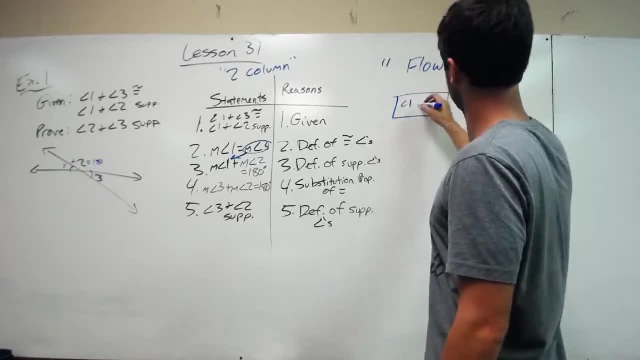 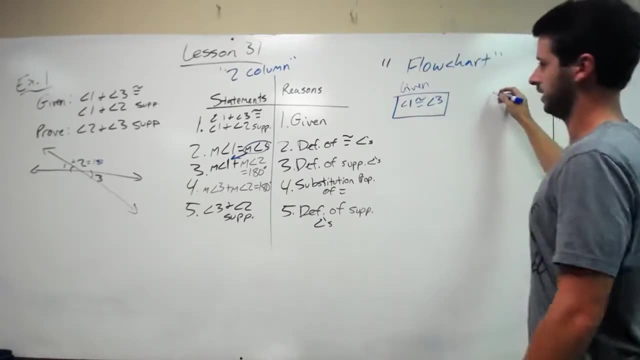 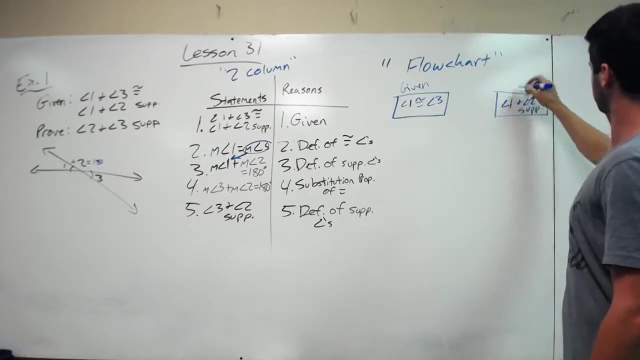 is say, angle 1 is congruent to angle 3. And that's a given. And then my other. I could also do this: Angle 1 and angle 2 are supplementary, And that's a given. So flowchart uses boxes. 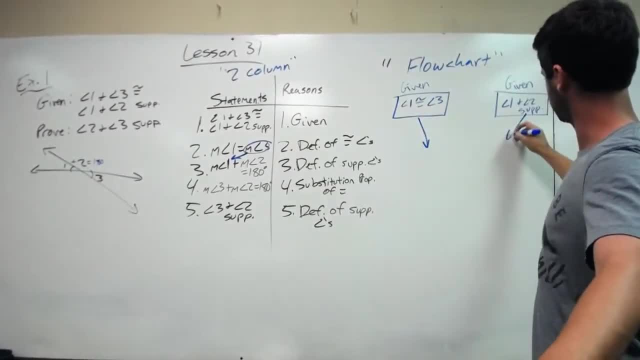 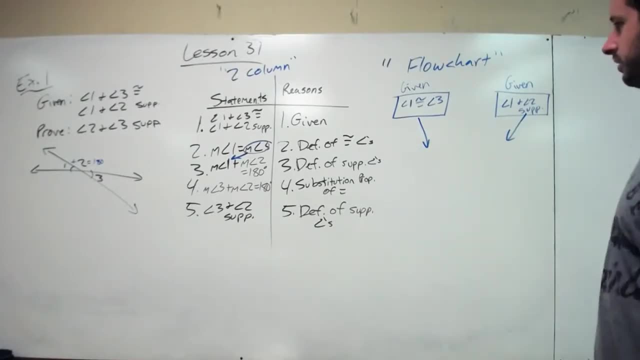 and arrows. So then, from here I take my next step, And it's read left to right, or top down is how you read flowcharts. So then my next part was: measure of angle 1 equals measure of angle 3. And that's definition. 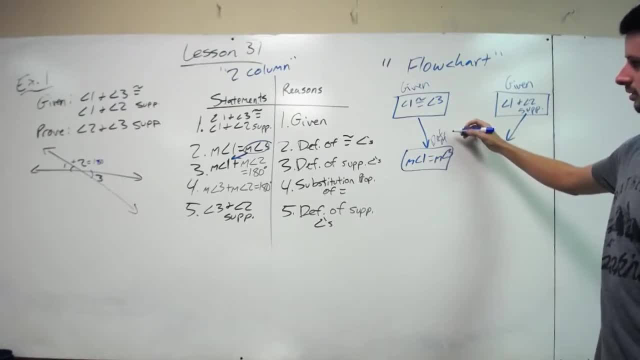 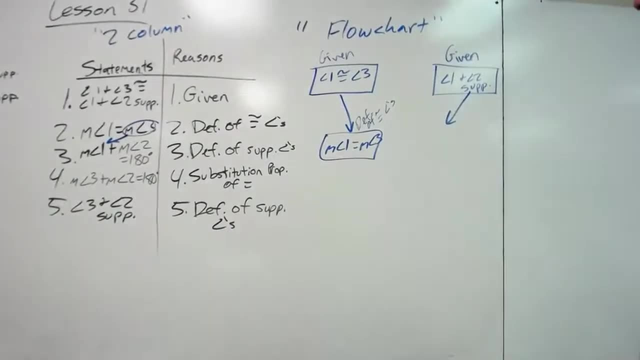 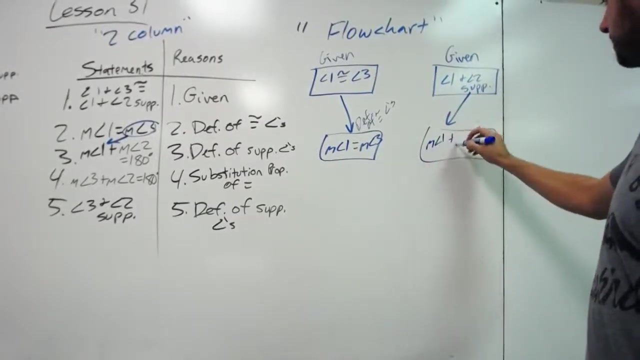 of congruent angles. It's going to be kind of small, but I'm trying to zoom in here. And then the other one was what went with. this was measure of angle 1 plus measure of angle 2 equals 180 degrees, And that's definition of supplementary angles. So you can kind of 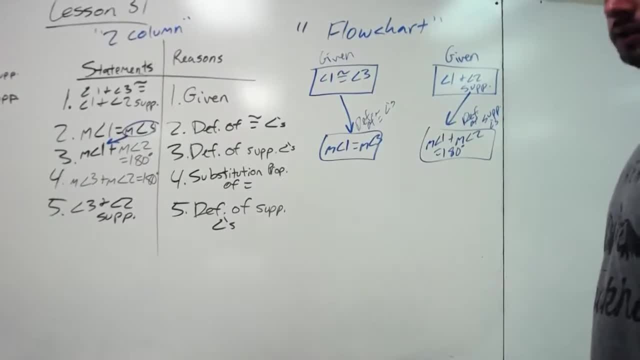 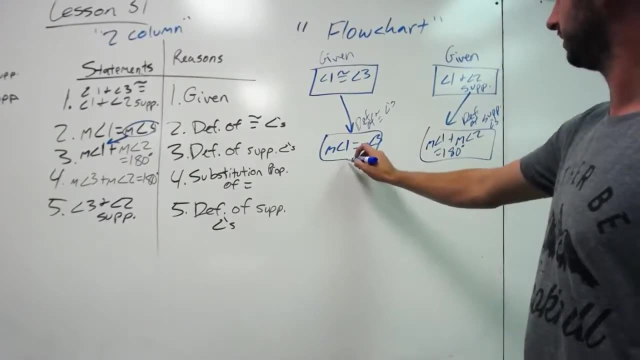 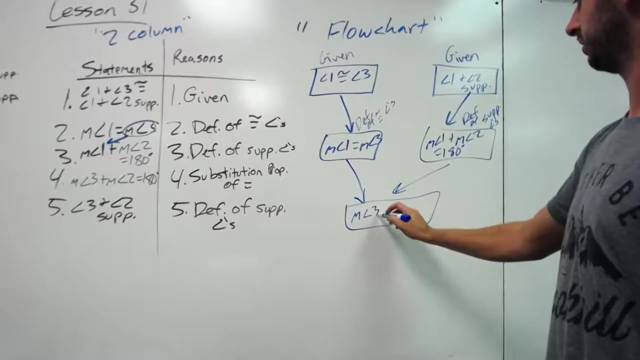 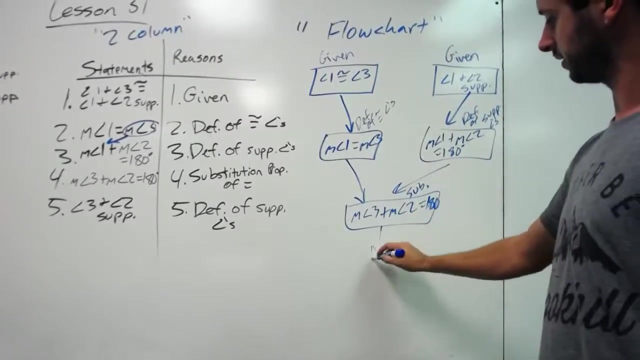 see the pattern. And then we have- let's see what can we do next, Angle 3, I could actually probably combine these: Measure of angle 3 plus measure of angle 2 equals 180.. And that's where I did substitution. 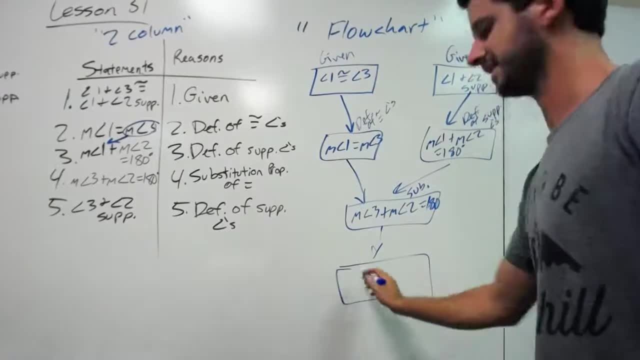 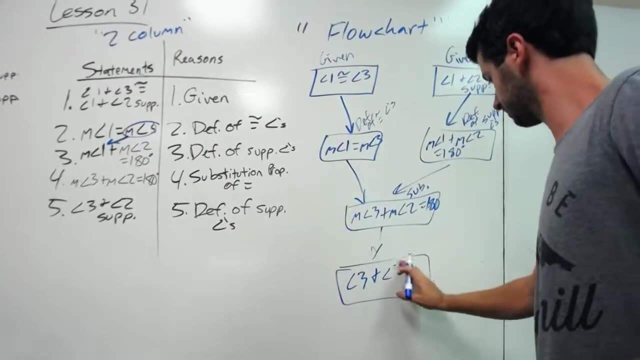 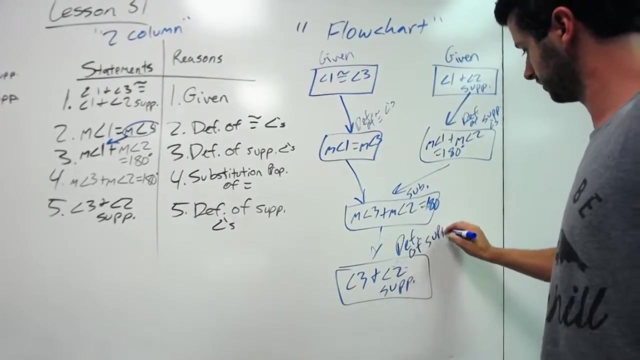 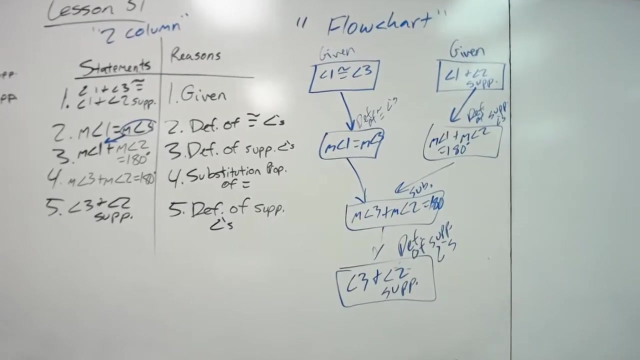 And then I could say the last thing I was looking for, angle 3 plus angle 2 is supplementary Definition of supplementary angles. So that is a flowchart style proof. The other type of proof that this teaches is the paragraph style proof, And I'm going 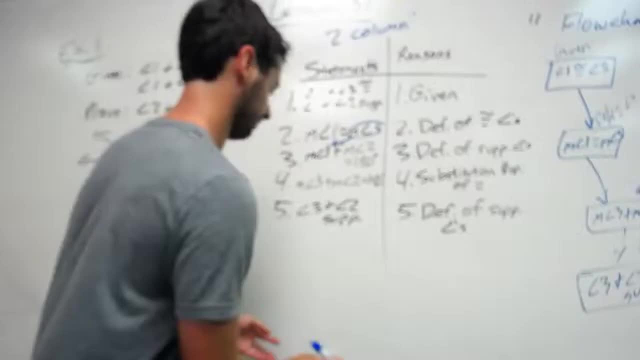 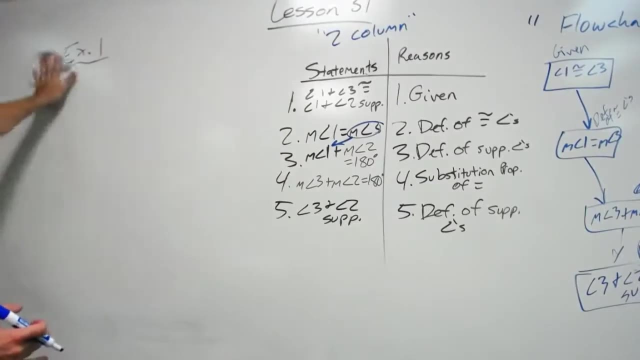 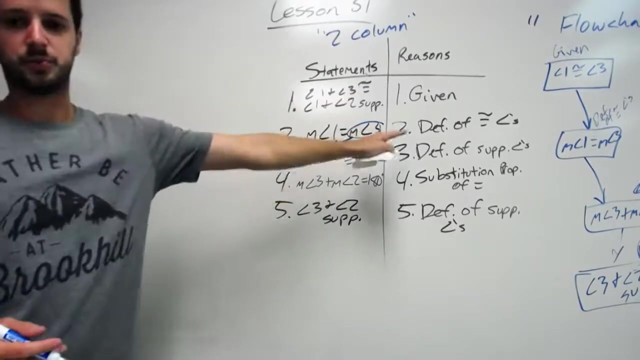 to erase this, because this really isn't what we're going for in this lesson. I'm just teaching you different types of ways to do it. I have had students liking the paragraph style Because what that would mean say we know our answer and we're just putting this in paragraph form.